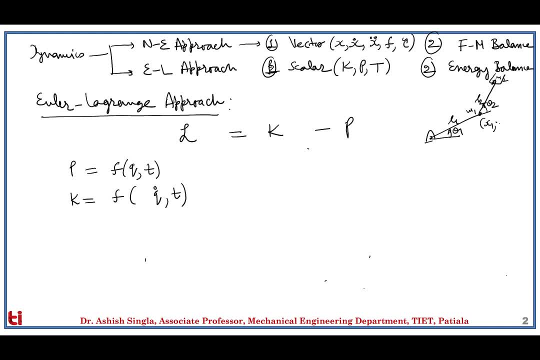 m1, m2. so the coordinates of the first link are, let's say, x1, y1 and the coordinates of the tip are, let's say, x2, y2. so we have x2 equal to L1, cos of theta 1 plus L2, cos of theta, 1 plus theta 2 and y2, we have L1, sine of theta. 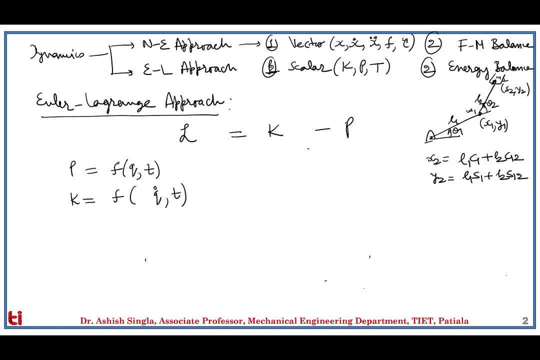 1 plus L2, sine of theta 1 plus theta 2. So let's take their derivatives. so we have X2 dot equal to minus L1. s1. theta 1 dot minus L2. s12 theta 12 dot where theta 12 represents theta one dot plus theta 2. 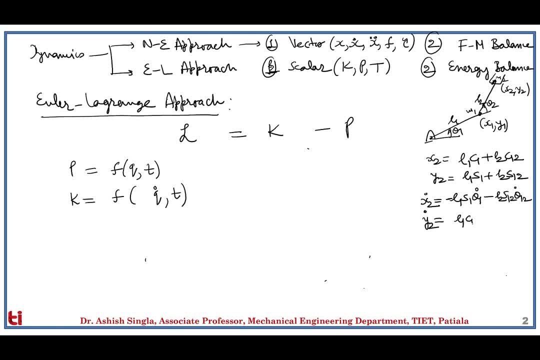 dot. similarly, we have Y2 dot equal to L1 c1- theta 1 dot plus L2 c1 one two theta one two dot. so now, in order to find out the kinetic energy of the body two, we need to take the square of this x two dot square plus y two dot square and multiply it by the mass of the. 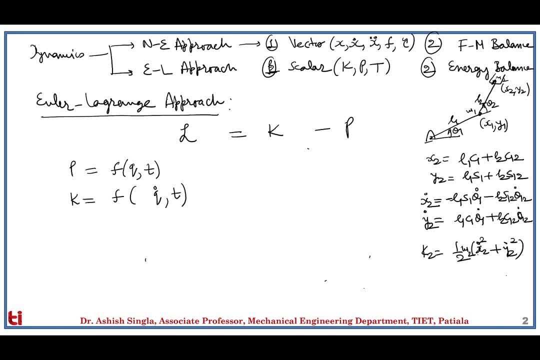 body two, that is, m. so here we can clearly see, because the kinetic energy contains the terms x two dot, y two dot, and both x two dot and y two dot are having dependence on theta one, theta two, theta one dot and theta two dot. so in nutshell we can say it depends upon q position. coordinates of 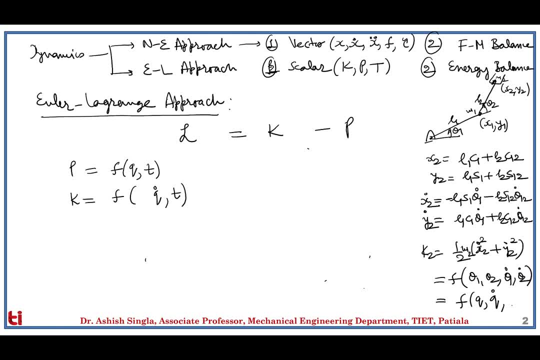 all the links and q dot the velocity of all the links, and also on t. so basically, the functional dependence of kinetic energy can be found here and we can write that the kinetic energy depends upon position, velocity as well as time. so that's why we can write this lagrange as q, q dot, t. 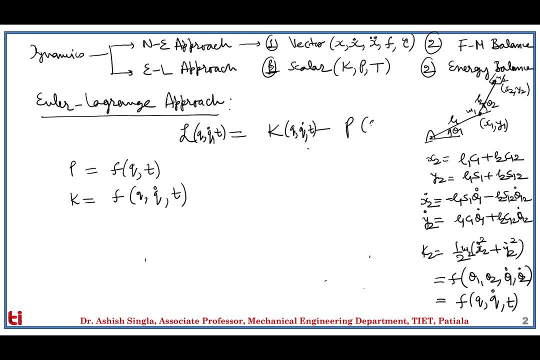 kinetic energy as q, q dot t and potential energy as q t. so this is the final result of this equation. So this is the functional dependence of each one of the terms. and finally we have the lagrange equation, which can be written as that: d by dt of del l by del q i dot minus del l by del q i plus del r by del q i dot equal to capital, q i, where i goes from one up to n, where n is the degrees of freedom of the system. 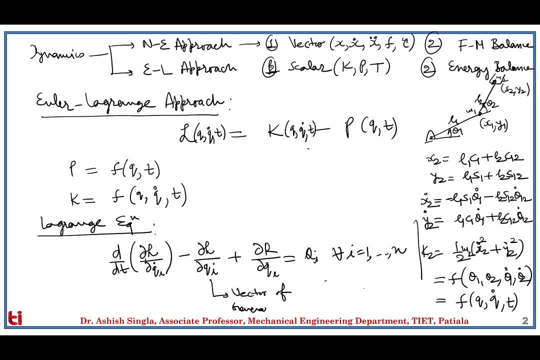 Here q i represents the vector of generalized coordinates, capital q i represents the vector of generalized coordinates, capital q i represents the vector of generalized coordinates, the vector of generalized forces, and this r represents Rayleigh's dissipation function and this r is responsible for all the energy being dissipated by the system. this may be because of friction, this may be because of air drag, this may be any other reason of damping. so this is called as a Rayleigh's dissipation function, which means that the total amount of energy being dissipated by the system 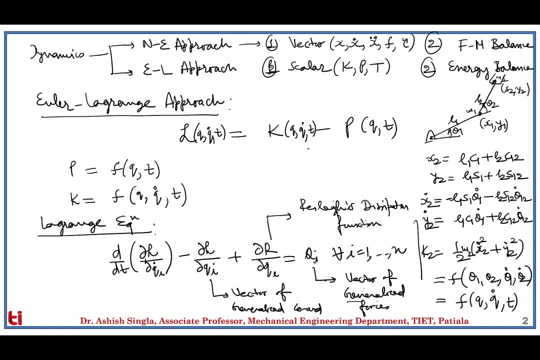 Next, we need to understand why we have used this special word called as generalized. Next, we need to understand why we have used this special word called as generalized Because, in Real life systems, most of our systems today are mechatronics. Real life systems, most of our systems today are mechatronics. 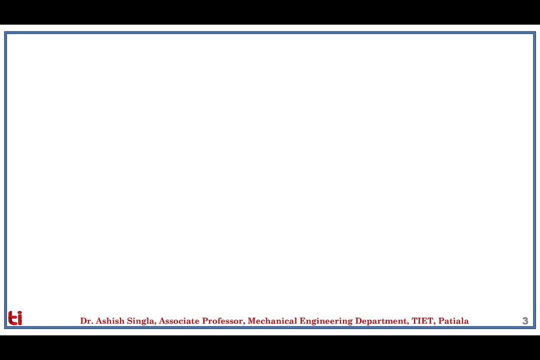 system which involves mechanical side, electrical side, electronic side, computer side. so in order to find out the overall transfer function of the system, we need to�: to study subsystem which may belong to mechanical domain, mechanical domain, electrical domain, electronics domain. to study subsystem which may belong to mechanical domain, electrical domain, electronics domain. so from each domain. 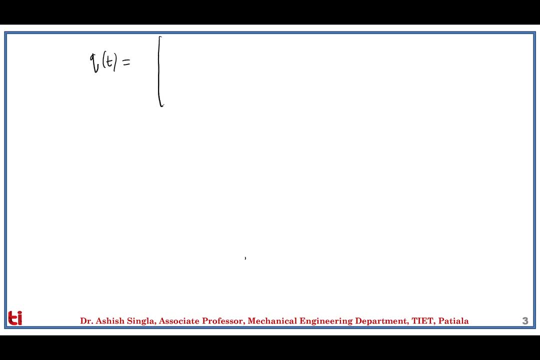 the vector Q. the vector Q represents the equivalent displacement variable. the vector Q represents the equivalent displacement variable. so it is in. let's say, if you're having a three degree freedom system where there are Transplantigen, and if you're having a three degree freedom system. 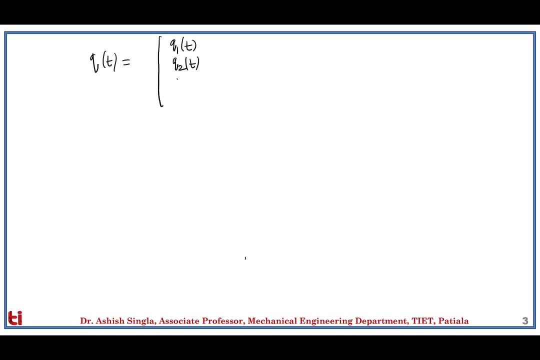 degree of freedom system. so it's q1, t, q2, t, q3, t, where q1, q2, q3, let's say, represents three different subsystems. so q1 may be having linear displacement, q2 may be rotary displacement and let's say q3 may represent the charge. so over here you can see all are representation of: 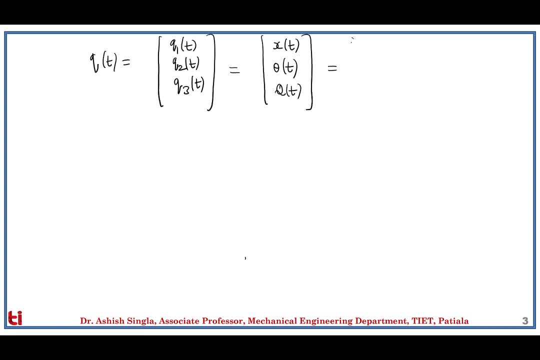 displacements and all three units need not to be same. so if we see over here, the units of xt are in meters, the units of theta are in radians and the units of charge are in ohms. even though all three units are different, but all three represents displacement in their 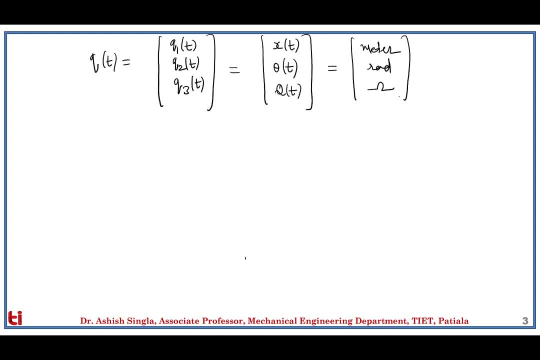 respective domains. that's why this q represents vector of generalized displacement. similarly, we have this capital q, which represents the vector of generalized forces. so, like the way we have, we can have a force, we can have a torque, we can have the emf, where we know the units of force are. 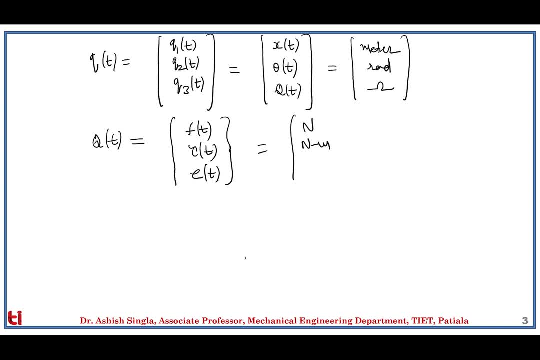 newton, the units of torque are newton meter, and then units of emf may be volts. now let's try to understand this euler lagrange approach with the help of one example. we'll take the same example as taken in the last session, and we'll try to see whether we have solved this problem using 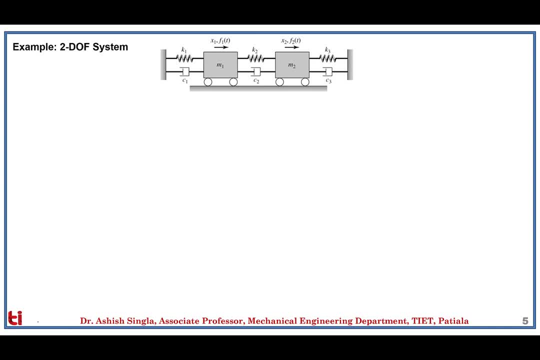 newton euler approach or by using euler lagrange approach, the dynamic model or equations of motion of this system will turn out to be same. so let's take this two degree of freedom system, where m1 and m2 represents the masses of two bodies and this system represents the masses of two bodies. 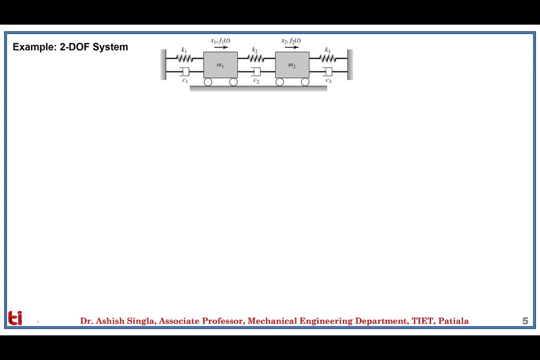 there are interconnected by three springs: k1, k2, k3 and three dampers, c1, c2, c3. so first of all, let's try to calculate the total kinetic energy of the system, which is equal to half m1 x1 dot square plus half m2 x2 dot square. then we have the potential energy of the system, the potential energy we know. 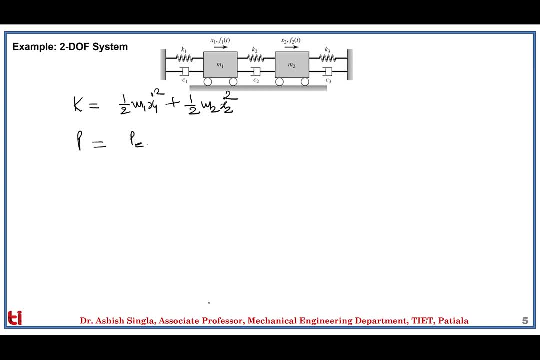 having two components: potential energy due to elastic deformation and potential energy due to the position of the body in the gravitational field. here both the bodies are lying on the ground, so we have only the elastic potential energy component, which is because of the amount of energy stored by each spring as strain energy. so we have half k1 x1 square because it's 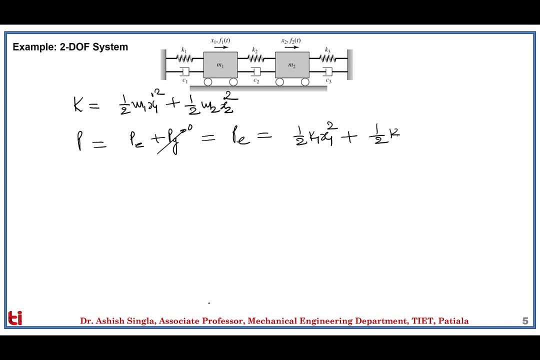 independent spring. one end is fixed. then we have half k2 x1 minus x2 square, because it's a coupled spring connected between both the bodies, and finally we have half k3 x2 square. so this is the total potential energy of the system and then we can calculate the 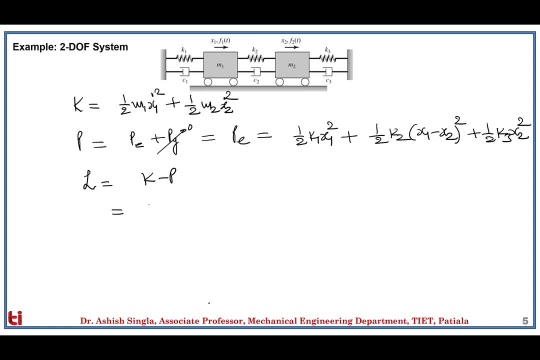 potential energy of the system, which is equal to half m1 x1 dot square plus half m2 x2 dot square, minus half k1 x1 square, minus half k2 x1 minus x2 square, minus half k3 x2 square. and finally we 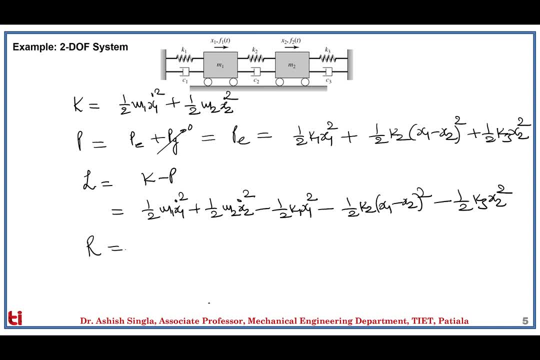 have the Rayleigh's dissipation function, which is equal to the total amount of energy being dissipated by the system. so it is equal to the amount of energy dissipated by the first system: half c1 x1 dot square, plus half c2 x1 dot minus x2 dot square, plus half c3 x2 dot square. so after: 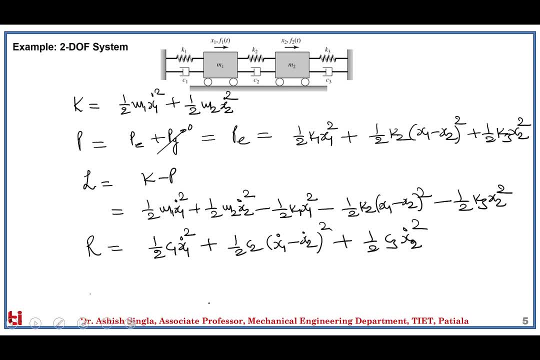 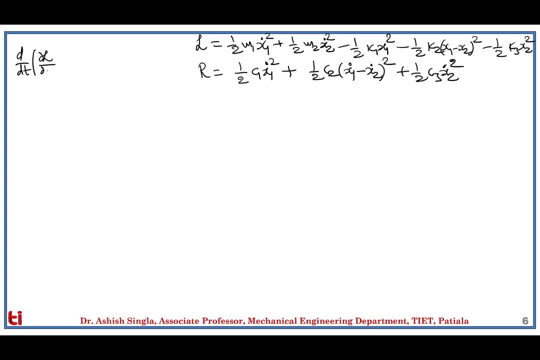 calculating these terms, we can now apply the Lagrange equations. so we have the Lagrange equation of del L by del qi dot minus Del L by Del qi plus del R by Del qi dot. equal to capital Ki. so let's take i index equal to one, and we know that the Q vector of generalized coordinates have q1, q2. 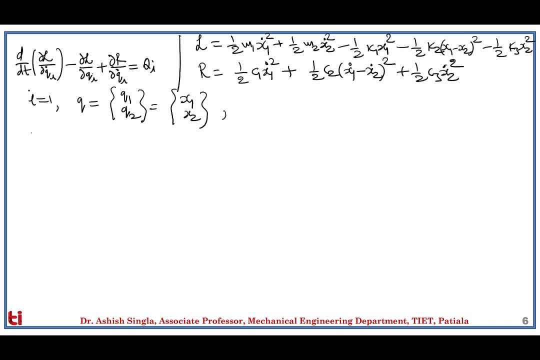 which is equal to x1, x2, so for i, equal to one we have q1 is equal to x1, so we can rented the x1 and z one and she will be at the point where x1 is equal to z1 and so we can arrenget this at point forward. and then let me legight this next first time so I thought I shouldn't remember Journey on the name, sum of two terms for the line action. I know the left fingers have two so we can go using game. we know that the right fingers in this problem our middle finger, the middle finger we can put on the top. 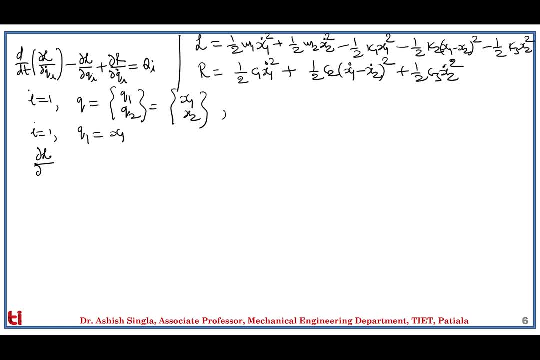 pathways and we need q and y hand for each one simultaneity Q and y hand. we have to loop our x1 and z two. we also. first of all, let's try to calculate del L by del x1 dot, which is equal to m1 x1. 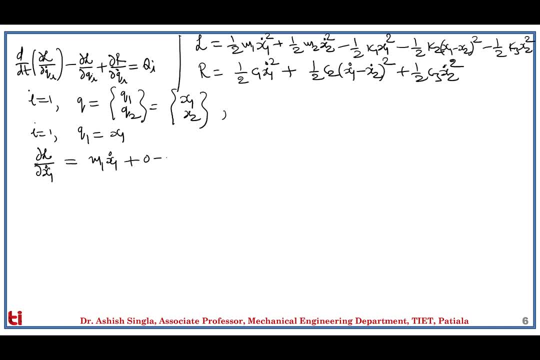 dot. then no contribution from second term, not from third, fourth and fifth. so next we have total derivative which is equal to d by dt of 4 del L by del x1 dot which is should be equal to m1 x1 double dot. then comes the second term. 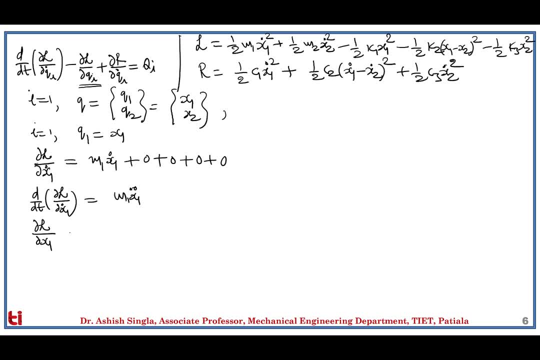 which is should be equal to del L by del x1. so if we see the Lagrangian, the first term does not have any X contribution: 0. second term again 0. third term depends on x1, so that's equal to minus k1 x1. fourth term also depends on: 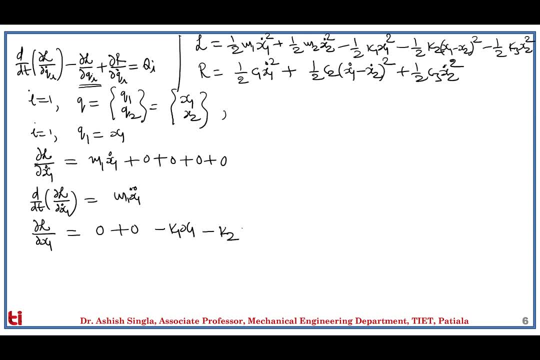 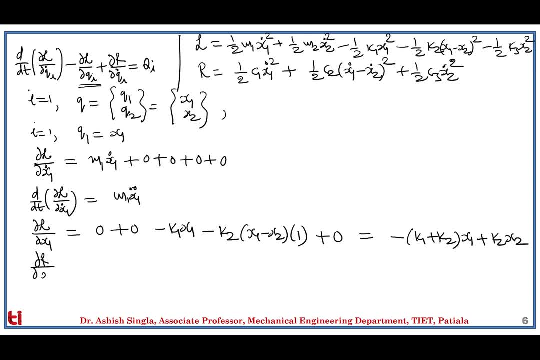 del R by del x1 dot, which can be written as c1, x1 dot plus c2 into x1 dot minus x2 dot into 1 plus 0, and it can be simplified as c1 plus c2 into x1 dot plus c2, x2 dot. and the q1 dot, finally, can be written as f1 of T. so we 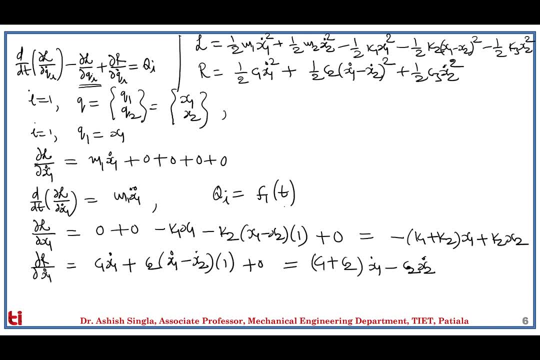 have evaluated all the terms. now we can plug in all these terms in the Lagrange equation, so that will give us m1- x1, double dot, minus dell L by del x1, that will give you plus k1 plus k2 x1 plus del L by del x1, that will give you plus k1 plus k2 x1. 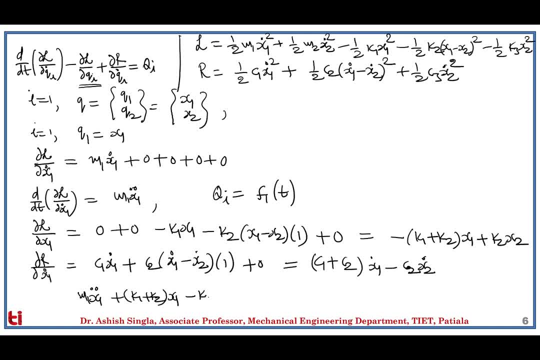 into x1 minus k2 x2. then we have del r by del q1 dot. that should give us c1 plus c2 times x1 dot minus c2. x2 dot equal to q1, that is equal to f1 of t. So this will give us the equation of motion of the first part. Now we can do the same steps. 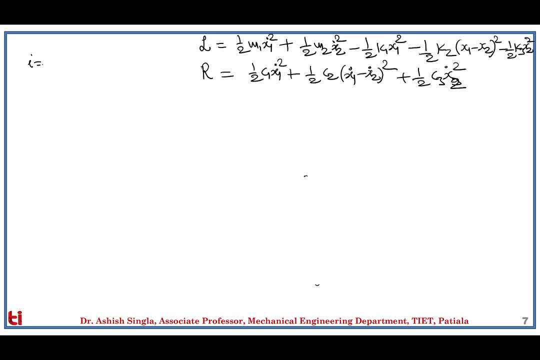 for i equal to 2.. So for i equal to 2. we know q2 is equal to x2.. So first of all we have del l by del q2 dot, which should be equal to del l by del x2 dot. that we can see the first term. 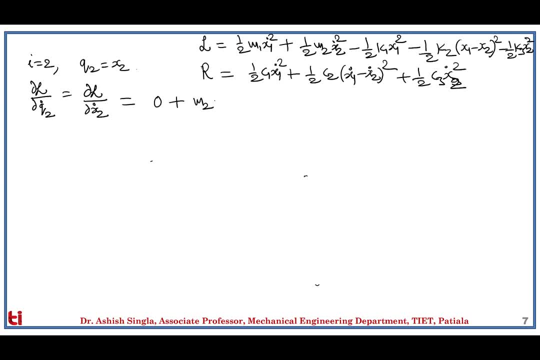 0. second term, we have m2 x2 dot and we have third, fourth and fifth term are also 0 because none of the terms are 0. So we will depend upon x2 dot. So next we have the total derivative d by dt of del, l by del x2 dot. 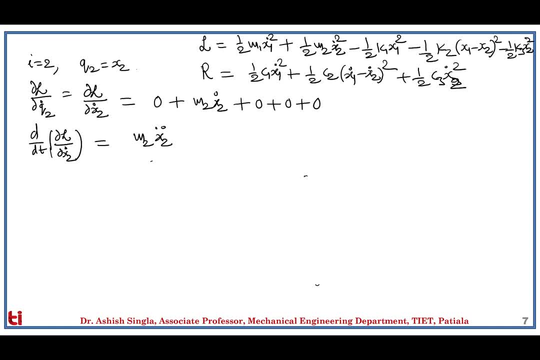 which is equal to m2 x2 double dot. Next we have del l by del x2, which should be equal to first term, 0 second term. we have 0 third term. also we have 0 fourth term. we have minus k2 into x1, minus x2.. 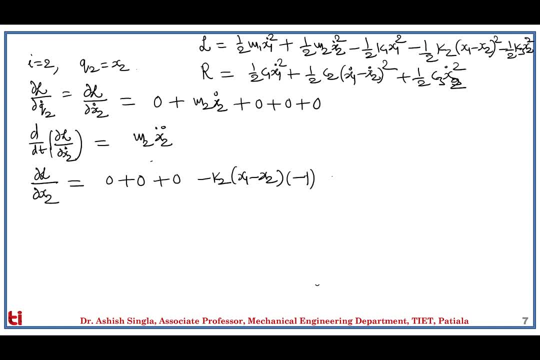 So we can simplify and combine the terms. So we have k2- x1 and then minus k2, plus k3 times x2.. So we can simplify and combine the terms, So we have k2- x1 and then minus k2, plus k3 times x2.. 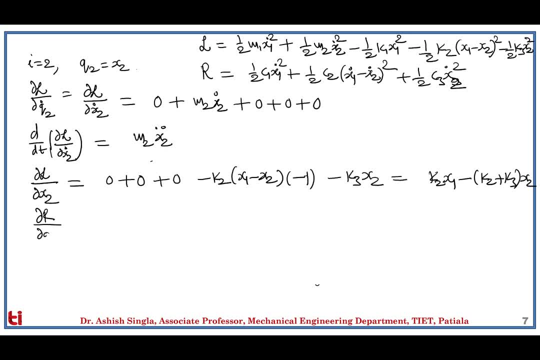 Next we have del r by del q2 dot, which is equal to del r by del x2 dot, which is equal to del r by del x2 dot. predicted term x1 is 0, which comes from index. same initial value is zero. ultimate return: 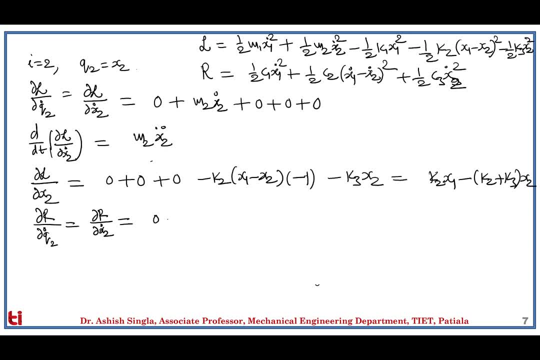 rate is zero and it can be written as: first term is zero. second term, we have c2 x1 dot, minus x2 dot and then minus 1, and finally, third term, we have c3 x2 dot, so which we can simplify and write as minus c2 x1 plus c2 plus c3 x2 dot, and finally we have normal. 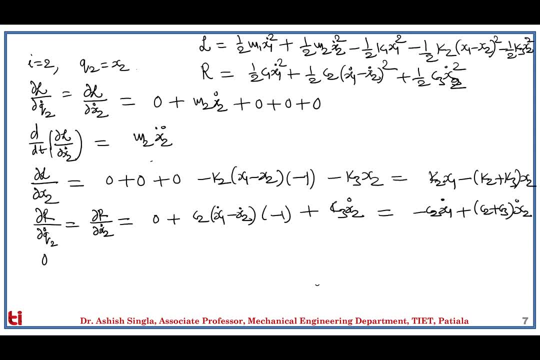 solution which is like that: 0. have. q2t is equal to f2. so again, we have calculated all the terms and we can plug in all these values in the lagrange equation, so which will give us m2x2, double dot minus k2x1 plus k2. 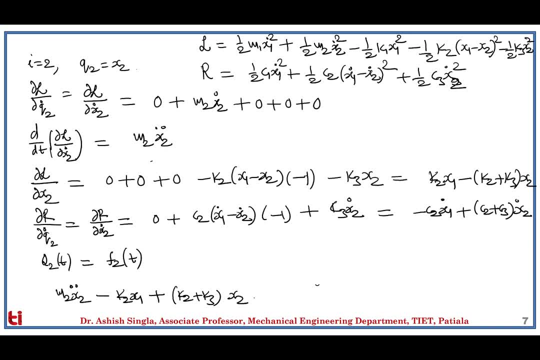 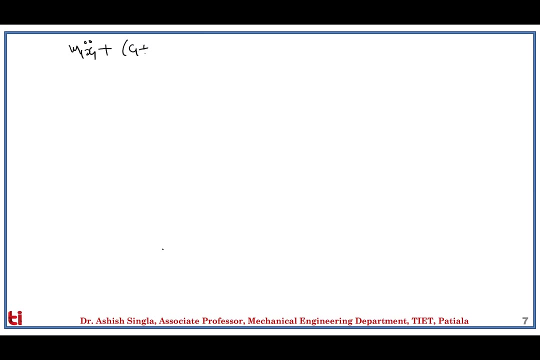 plus k3 times x2 minus c2x1 dot plus c2 plus c3 x2 dot should be equal to f2. so this is the equation of motion of the second body. so we have the first equation as m1x1 double dot plus c1 plus c2 times x1 dot minus c2x2 dot plus c2x1 dot plus c2x1 dot plus c2x2. 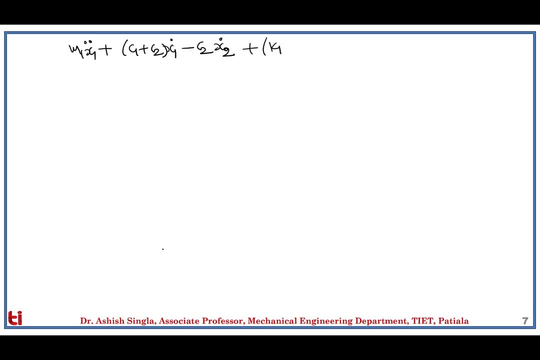 dot. then we have k1 plus k2 times x1 minus k2x2, equal to f1 of t. that is first equation. and then we have the second equation as m2x2 double dot minus c2x1, dot plus c2 plus c3. 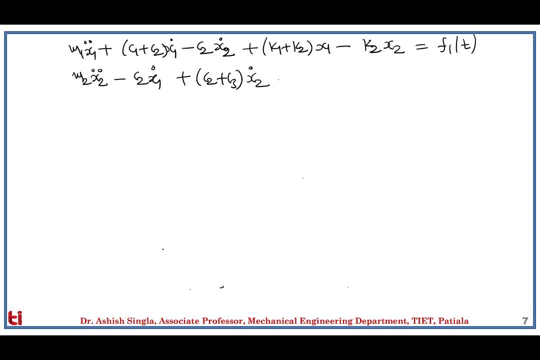 times x2 dot. then minus k2x1 plus k2 plus k3 times x2 is equal to f2. now we can write this in matrix forms. so where the structure of equation is mx, double dot plus cx, dot plus kx should be equal to f of t, so where x represents the vector of generalized coordinates. so we have: 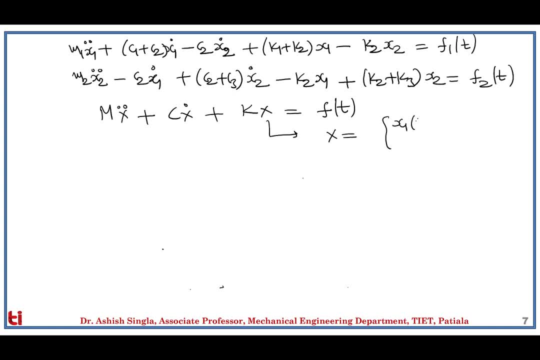 some part or this will come. that is this and will come: x1 dot, x2 dot. then we have x1- x2, which should be equal to f1 t, f2 t. so if we now see the first equation- and we will try to write this in the as the first row of this matrix so we can see that- 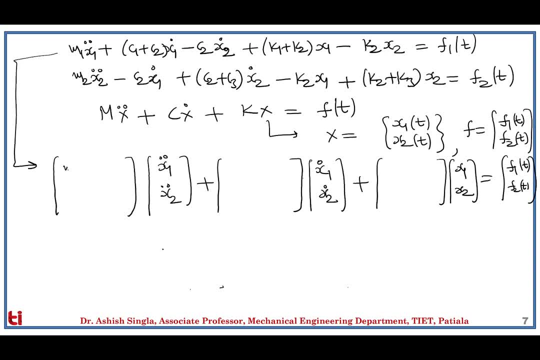 there is contribution from x1 double dot, so that will be m1, but there is no contribution from the x2 double dot, so that entry is 0. so next we have x1 dot, which is equal to c1 plus c2, and x2 dot. 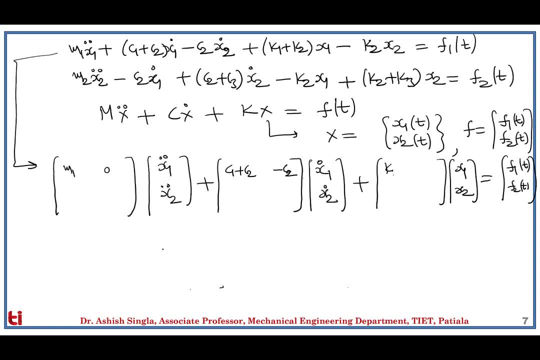 is minus c2, then we have k1 plus k2 for x1 and then minus k2 for x2, and then f1 is over here in the right hand side. similarly, now we can go to equation number 2. so we can see that from the equation number 2, which 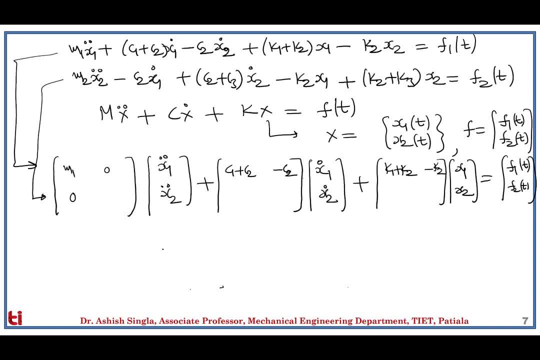 should come as second row. so there is no contribution from x1 double dot, m2 for x2 double dot. so then we have minus c2 times x1 dot, c2 plus c3 times x2 dot, and then we have minus k2, k2 plus k3. so this is the dynamic model in matrix form. we